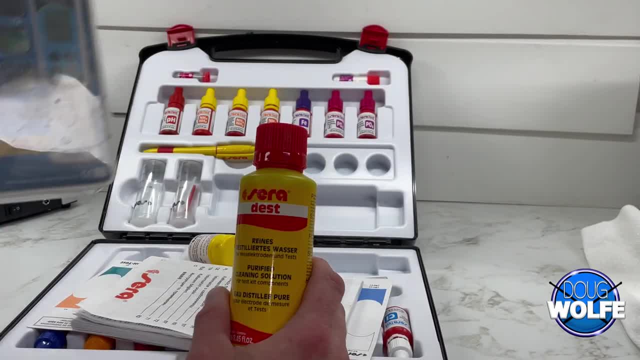 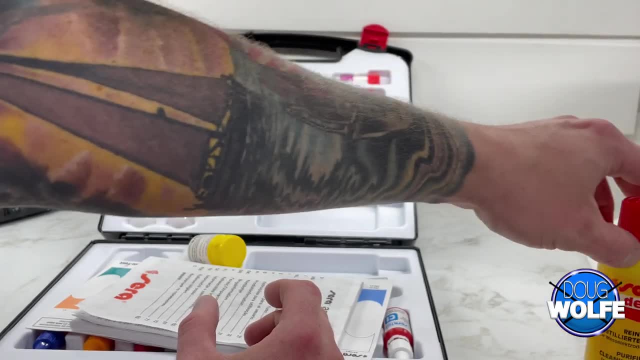 equipment. if you have like a pH meter or something, you can rinse your electrodes with it. You don't want to rinse that type of stuff with tap water because it's conductive and you don't want conductive water when you're doing that. So, anyways, this comes with. 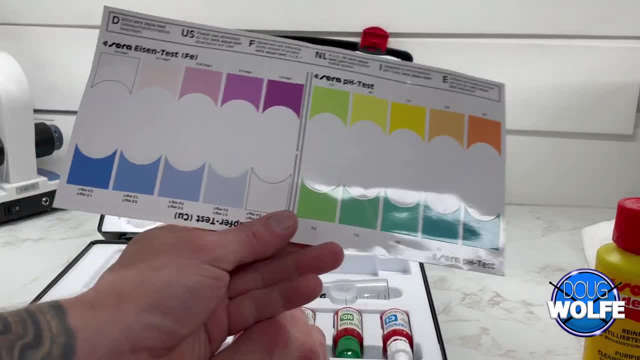 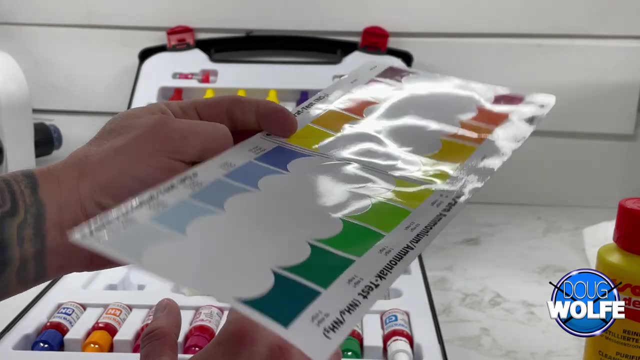 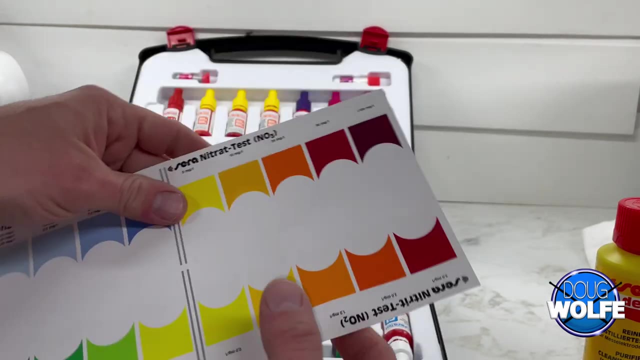 tap water Typical instruction booklet. And this is: this is one of the things that I like the most about this kit: It's laminated for one so it doesn't get wet, And it has a good color spectrum on all of these tests So, for example, your nitrate, you actually have a good range where you can get an. 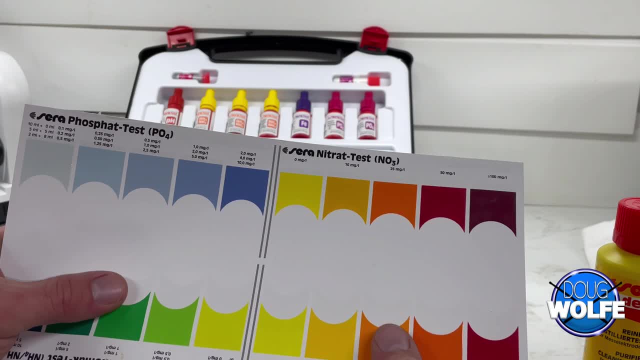 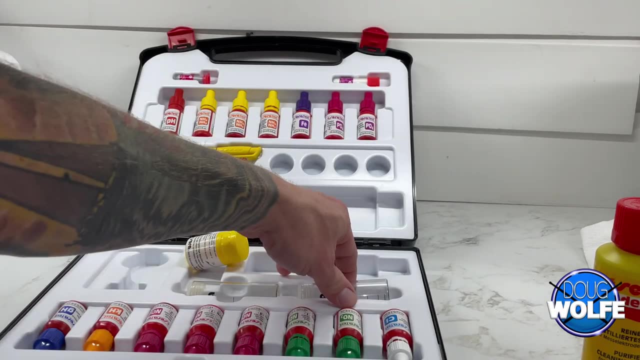 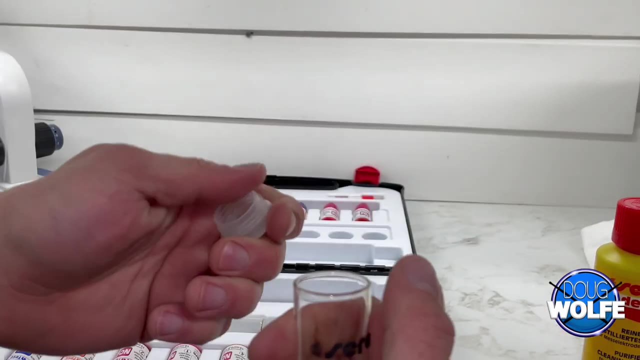 accurate reading and not just this dark red to blood red where you really can't tell the difference. So this is probably one of my favorite things about the kit: That, in addition to the actual test vials themselves are super thick. They're larger than other vials that you would receive Nice thick. 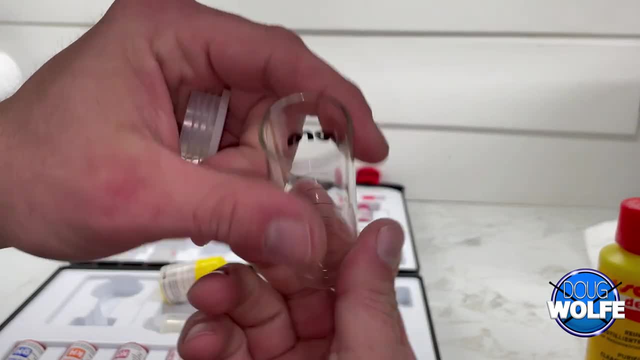 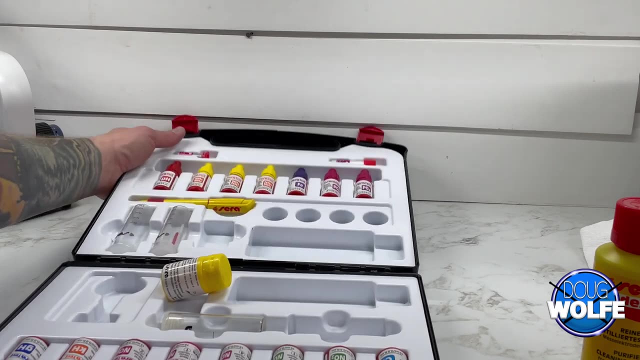 glass. They're not going to break easily. I need to clean it a little bit better, But this is a great- another great aspect of the test that I do like. So it does come with the following: This kit is around 80 or $90.. 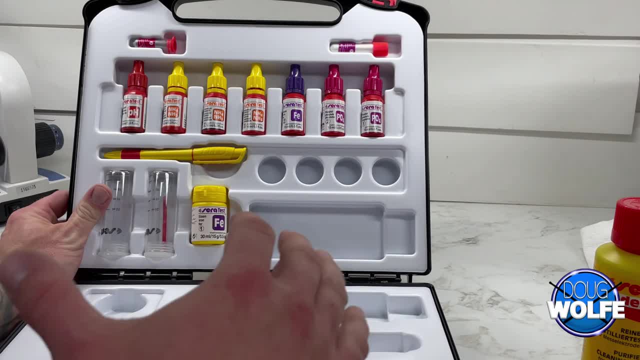 Um, which seems a little bit higher than some of the other kits, but, uh, for what you're getting out of it And I think you'll see that, uh, my dog is barking. I'm sorry, I think that you'll see. 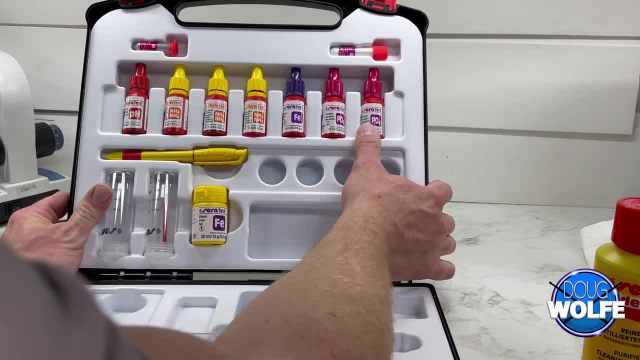 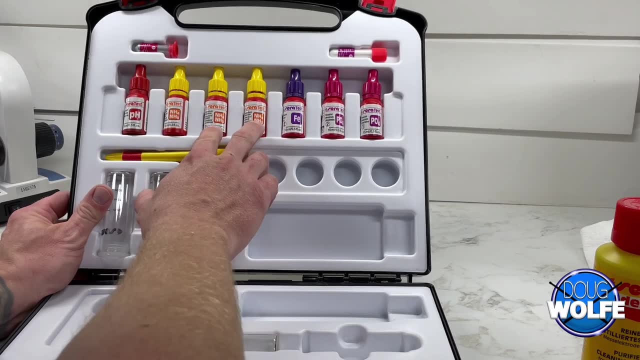 uh, that it's worth the money in the long run. So it comes with phosphate test kit. It comes with iron test NH4,- NH3 is your ammonia, There's three of those- Your pH And this is also part of the. 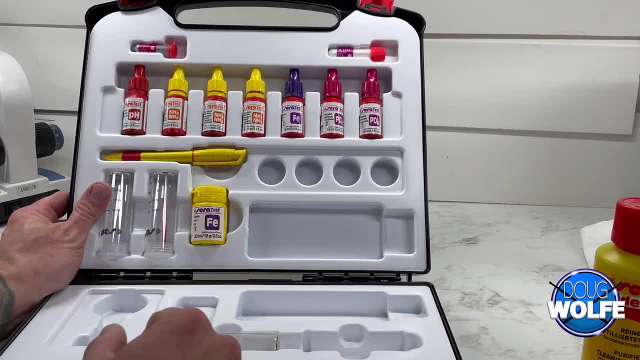 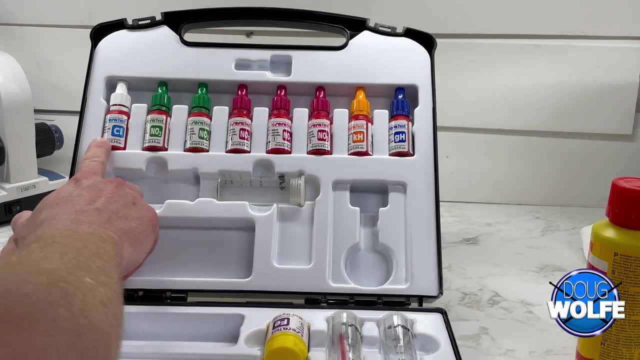 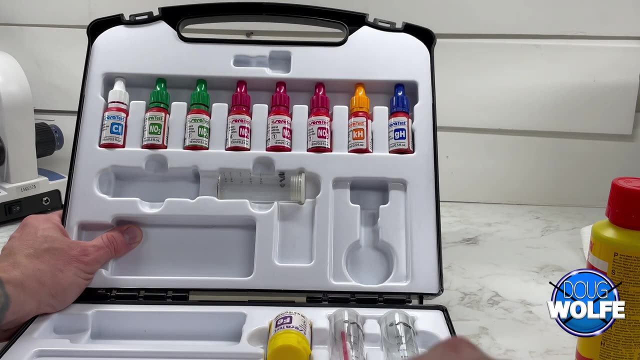 iron test. It comes with four uh test vials, A nice pen And on the other side here got chlorine test- NO2, your nitrites, NO3, your nitrates- There's three of them And actually uh another, another little uh region that we'll get. 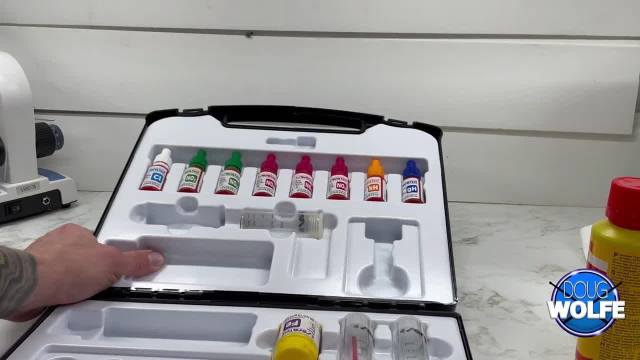 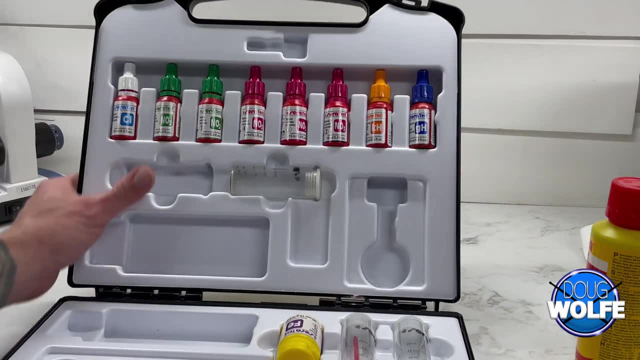 to. And then your hardness, KH and GH, Um overall. just to give you a quick summary, I think this test kit is superior to um- at least the two others that I've tried- So I'm going to be giving any any manufacturer. 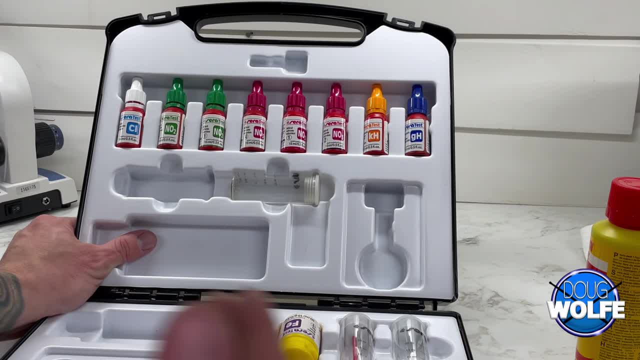 try, uh, just to see you know how they vary from one to the next. uh, the ease of testing, how long it takes to test how well the kits put together. Um, the results obviously, is the most important thing, but, uh, the other other things that we'll touch on, uh, as I'm going to do these, 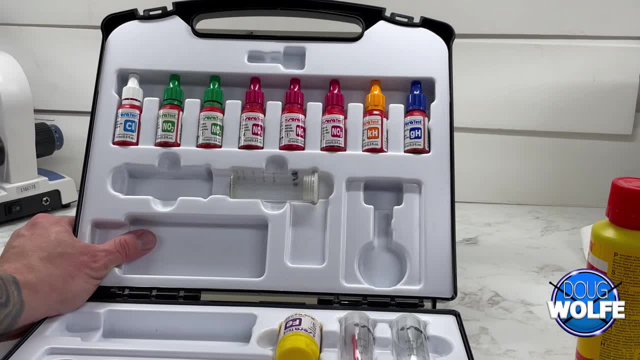 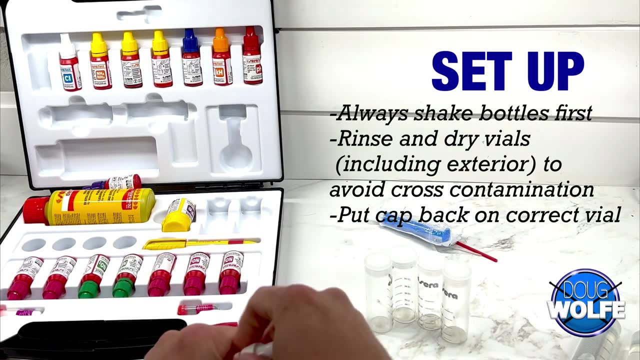 tests right now, but overall I would definitely recommend this. That's my quick answer. Um, so far it's the best test kit that I've used. When you initially open these, you have to take the point of the cap And pierce this, All right. So it says for all these tests, to make sure you shake the bottle well. 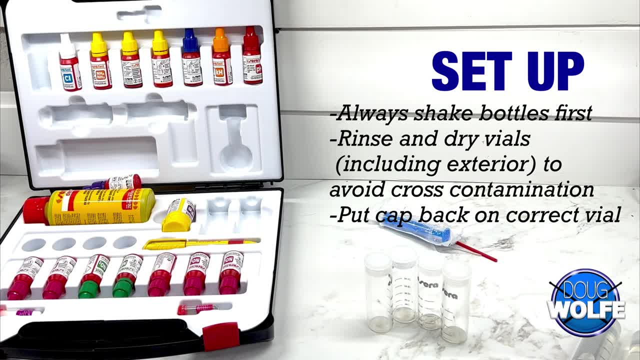 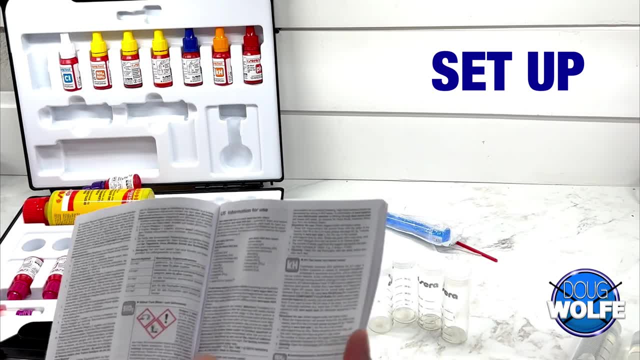 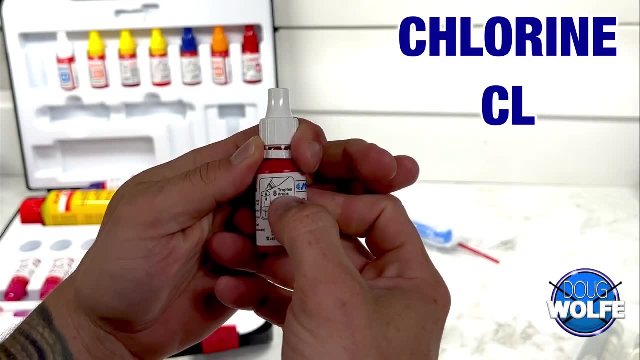 first, So we'll do that Now. it does tell you um on the instructions how to do each of these tests. Okay, The first test we're going to do is chlorine: 10 milliliters, eight drops right. 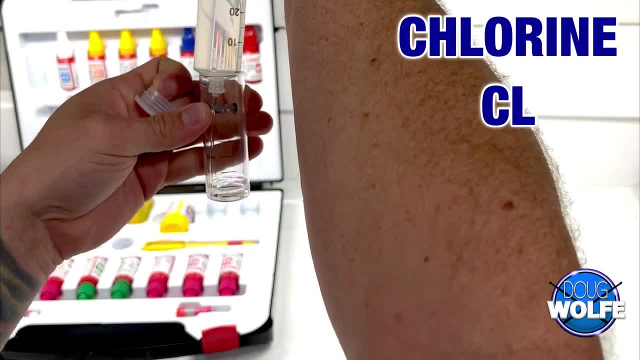 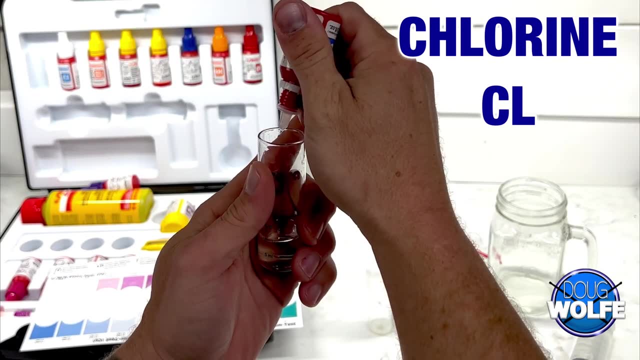 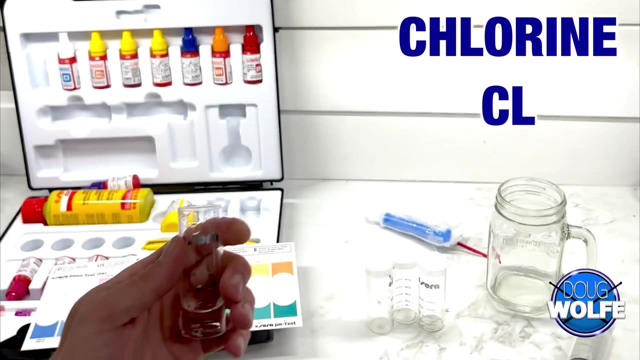 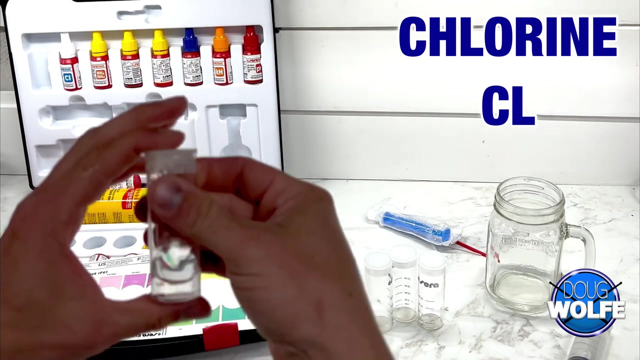 So I've already done that, I've already grabbed the tank water to speed this up: One, two, three, four, five, six, seven, eight, Shake it And basically you want to do this in very well lit conditions or daylight, Um, and this would start changing. So I'm going to do this in very well lit conditions or daylight Um, and this would start changing. So I'm going to do this in very well lit conditions or daylight Um, and this would start changing immediately. Um, and this would start changing immediately if there was chlorine in it. 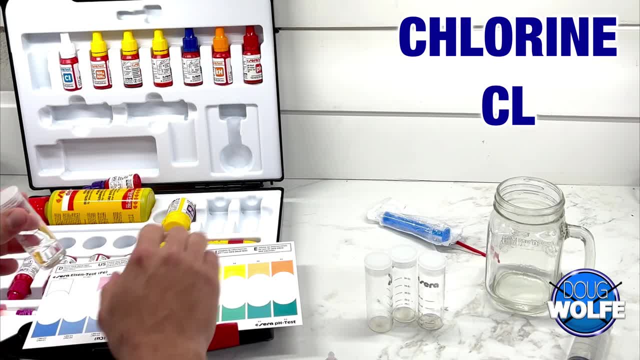 changing immediately if there was Chlorine in it. um, so there's not anything really to compare it to. um, so there's not anything really to comparison. um, so there's not anything really to compare it to before. it caused a change. and it does say um, and. 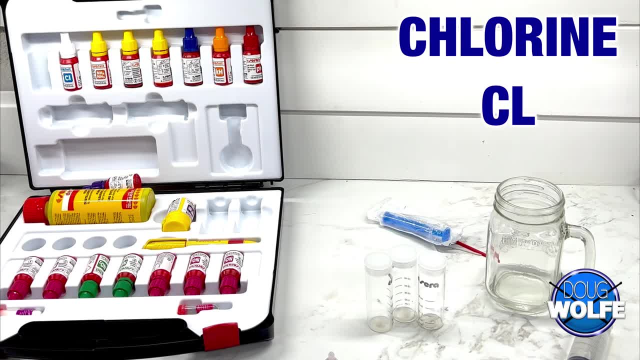 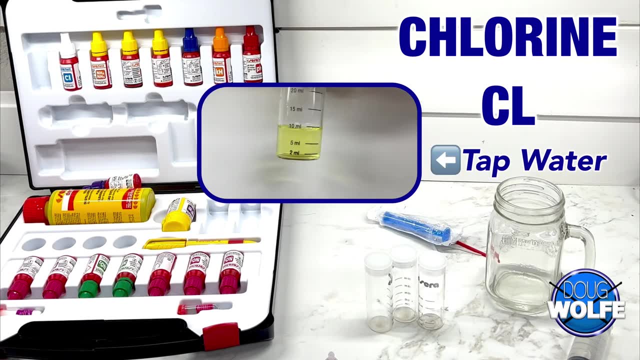 if no color change occurs, this water is chlorine free. Great meaningful chlorine levels from point O. two milligrams leader will establish a yellow coloration with higher. has a yellow coloration with higher chlorine levels. become greater colorization with higher. So as you can see, we're good, no effect. 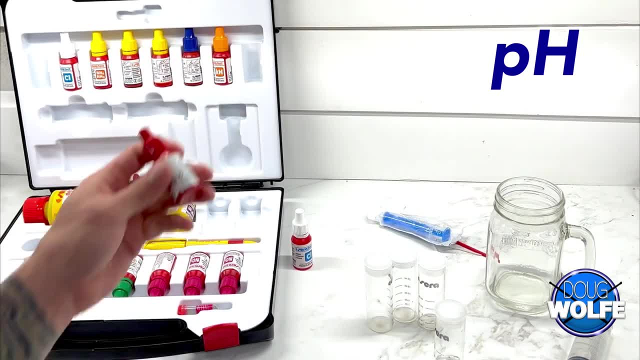 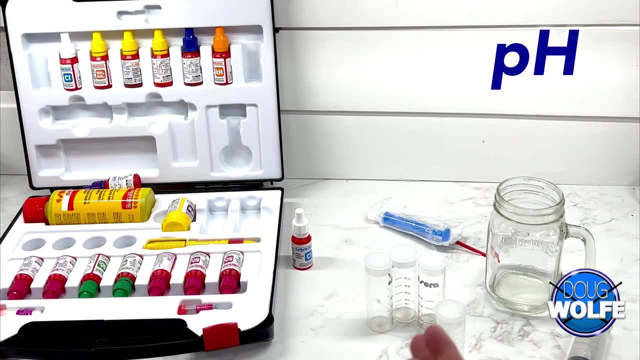 somethin cooler, because it's what is ph? uh, and what i like about this ph test is it's just one bottle. it's not high ph, it's not low ph, not trying to figure out that gray area in the middle. um, just one ph test, so that's awesome. 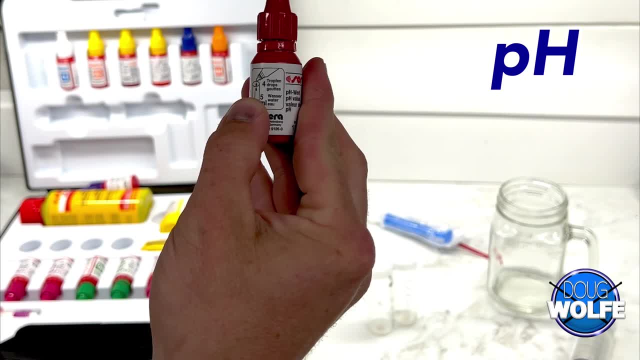 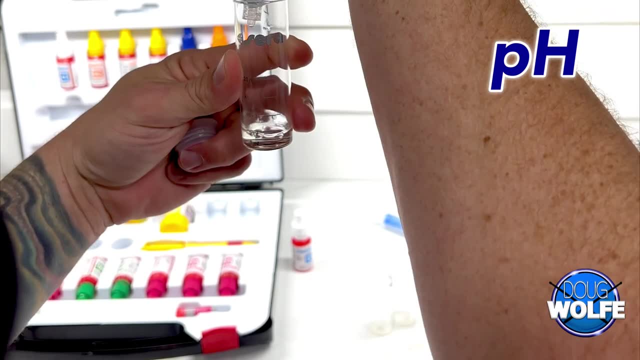 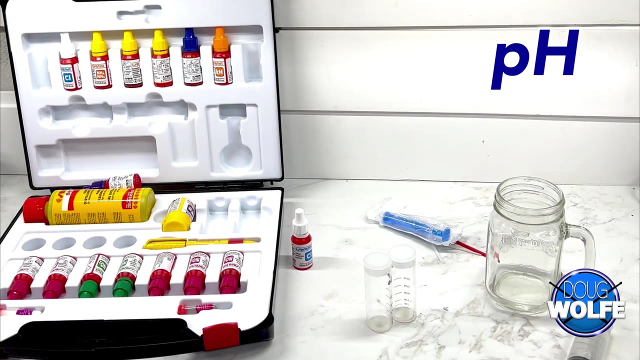 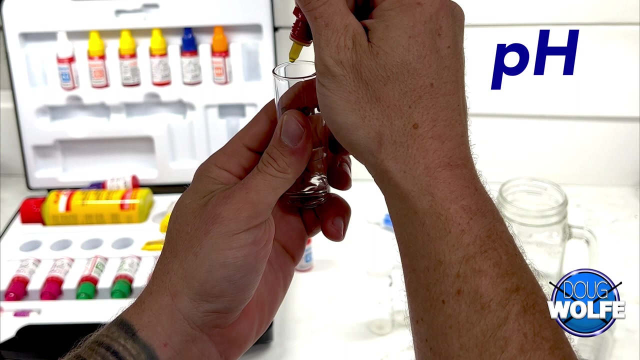 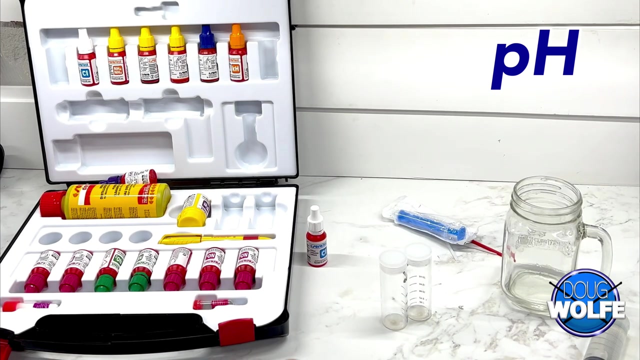 okay, so for ph we are going to do four drops into five milliliters: one, two, three, four. i'm sorry i have to count out loud or i forget how many drops. i do guaranteed you just shake it till the color is clear and then you're good to go. 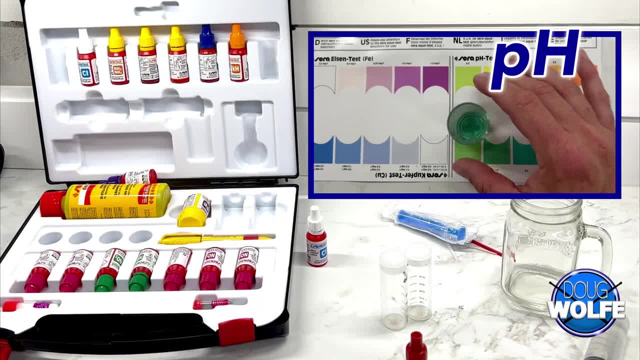 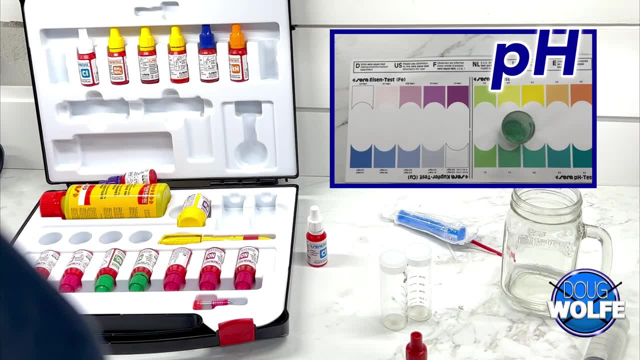 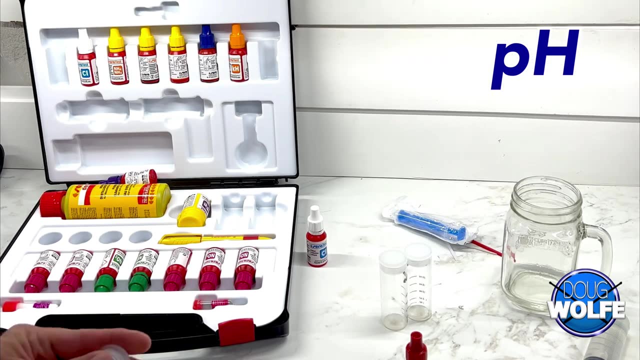 uniform till it's all mixed in. then you go down and you sort of line it up with where you're at. so i am somewhere between seven, five and eight, which is where i want to be with this tank. so we're going to do the nitrite testing- two bottles. 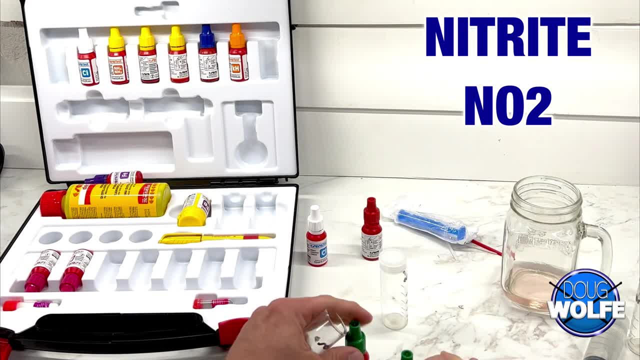 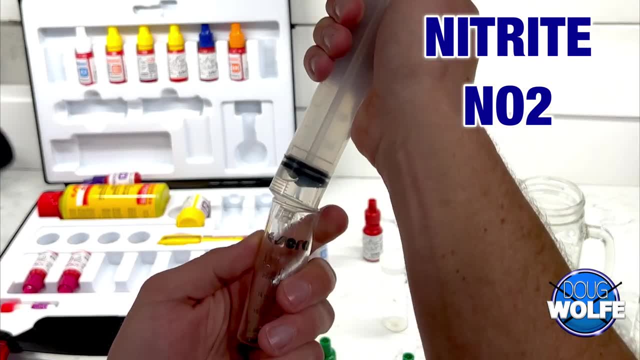 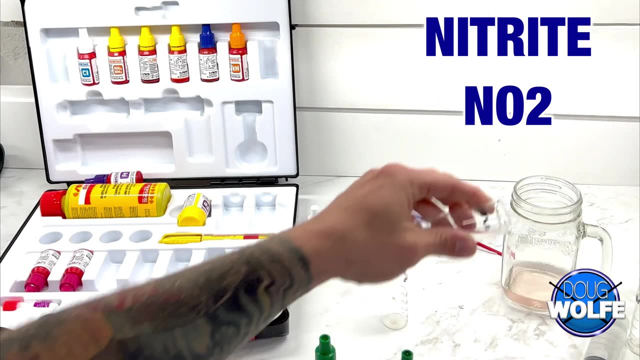 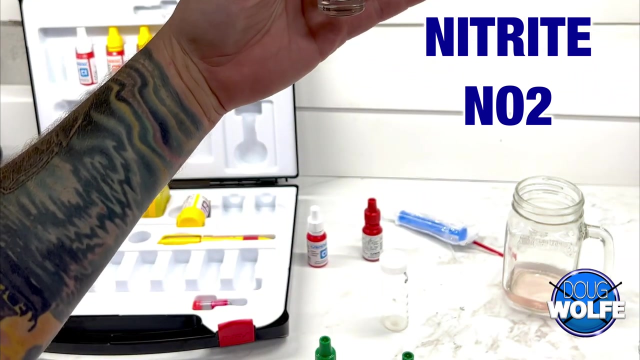 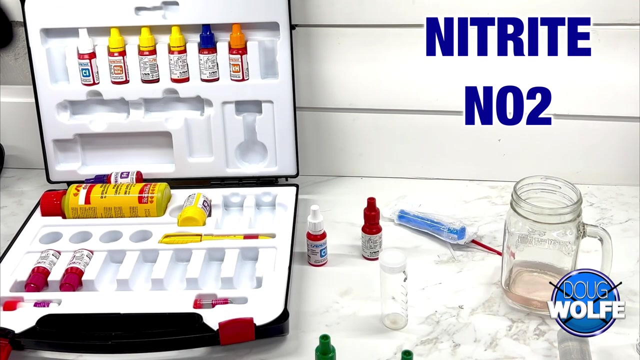 so we're going to need five milliliters and five drops. one thing i noticed about this test is um. i couldn't find very many um videos about this, this product in in english or in the united states. most of them were um overseas somewhere. so hopefully this is beneficial to somebody. but anyway, all right, five. 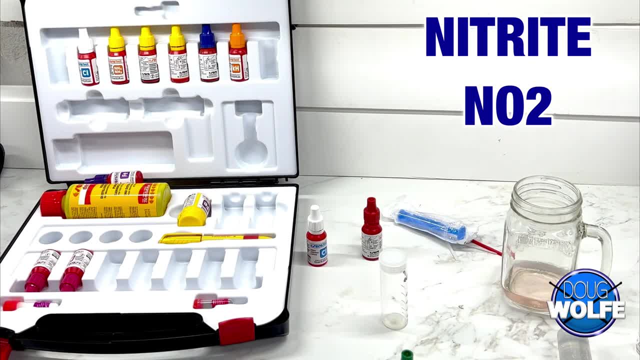 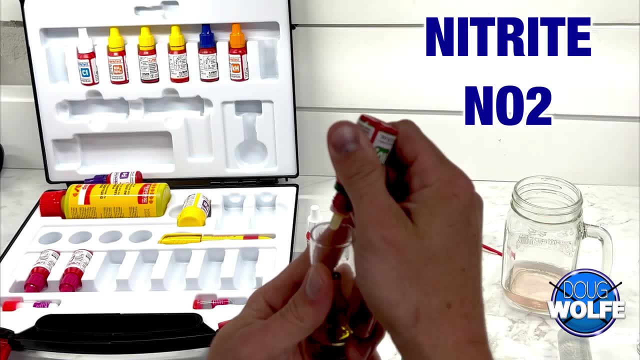 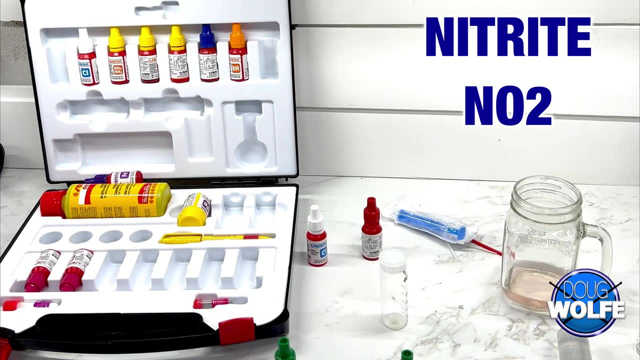 drops one, two, three, four, five. one thing i love about this test kit is the drops come out very uniform and consistent and it's not like if you squeeze it too much or too little. um, with some, like some other test kits, you know you get 30 drops and you're only meant to have two. 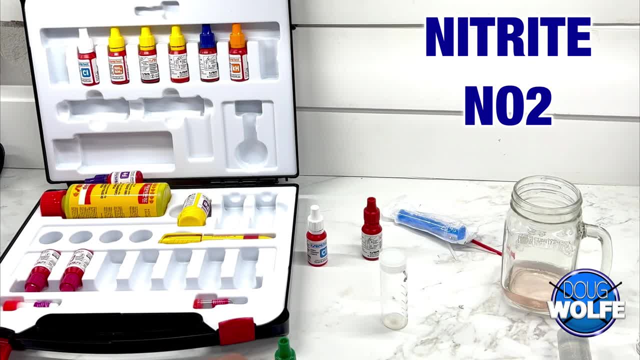 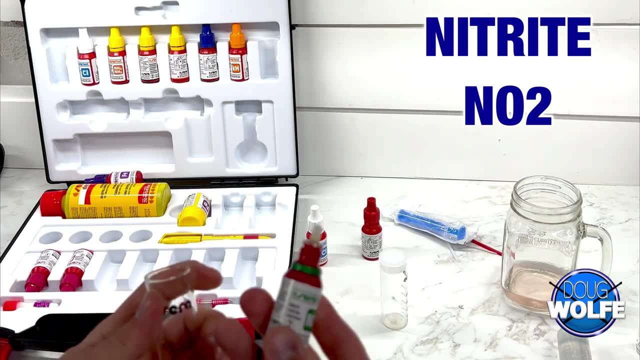 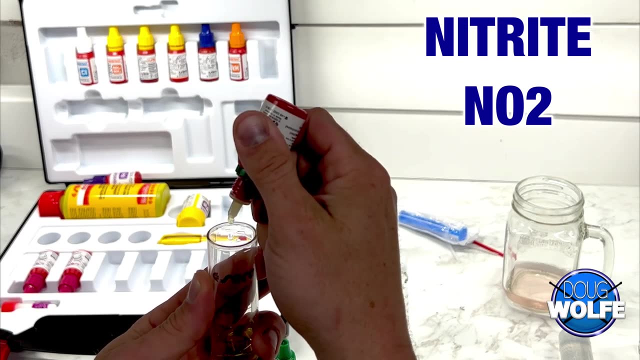 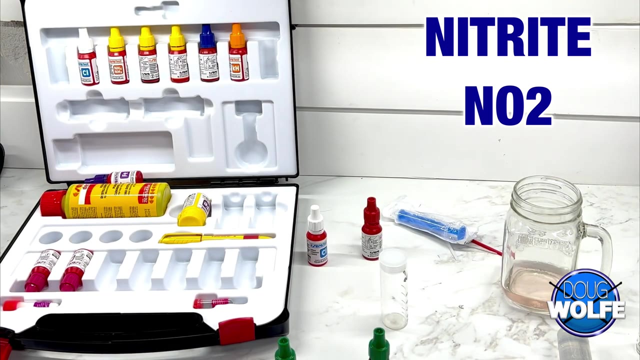 i don't really have that problem with this kit. i also really like the fact that for the most part you know your instructions and what you need to do or right on the bottles. you don't have to keep referencing the, the booklet, same thing: one, two, three, four, five. shake it not for any length of time, just until everything is. 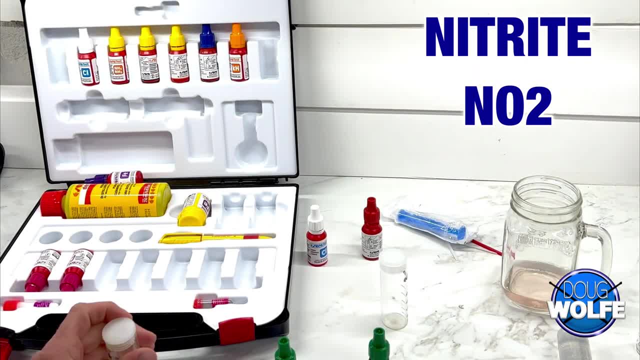 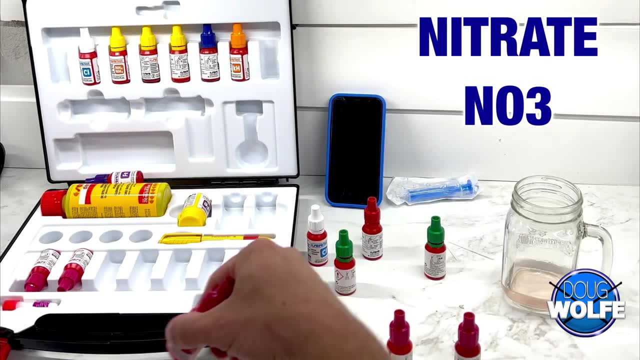 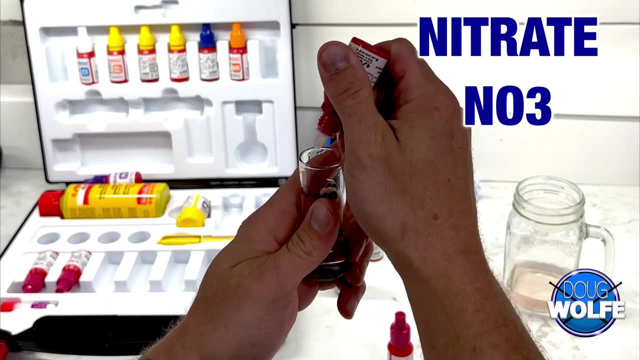 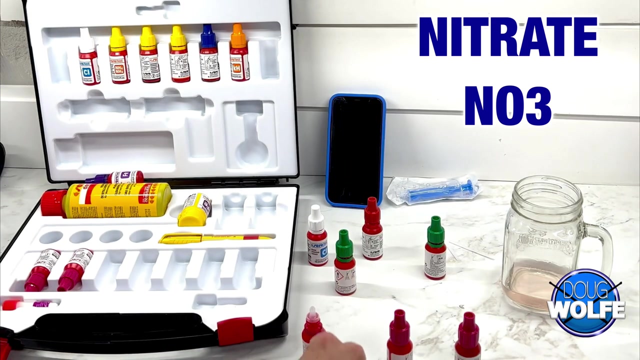 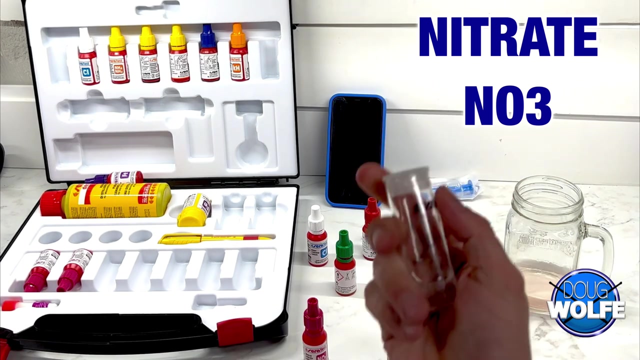 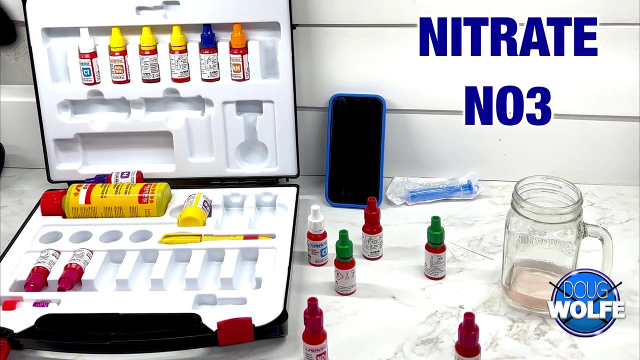 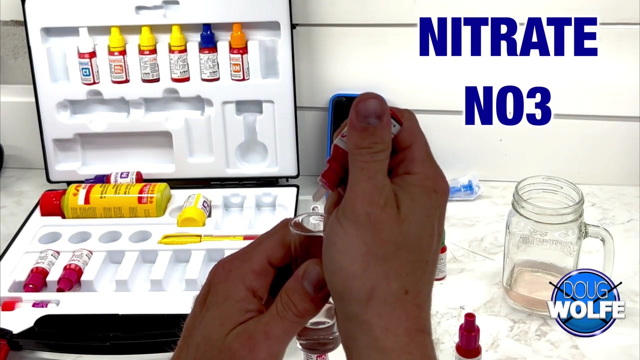 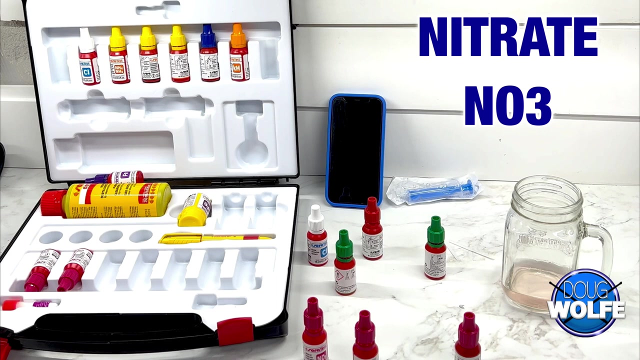 mixed together. good, so timer for five minutes. then we'll come back to this. one, okay, six drops ten milliliters. one, two, three, four, five, six and cap it and shake it. okay, bottle number two: six drops ten milliliters. one, two, three, four, five, six. 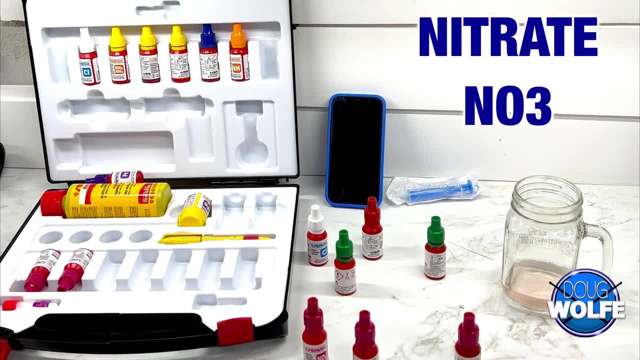 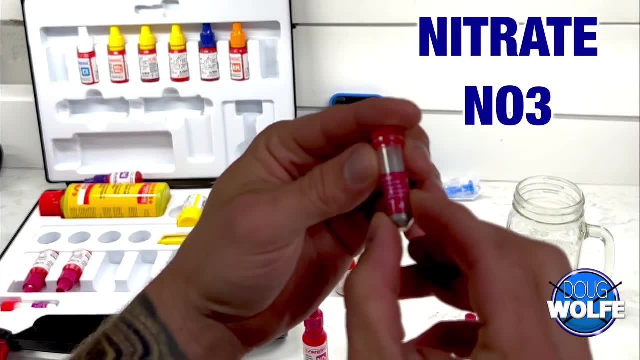 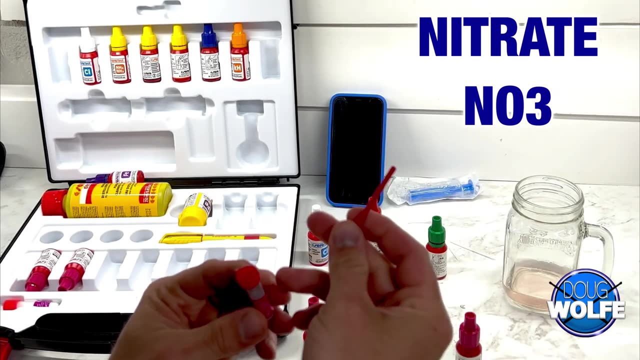 same thing. okay, now for three, we are going to use this little um tube here and this uh spoon- i guess you would call it a spoon- and then we're going to use this little um tube here, and then we're going to use this little um tube here, and 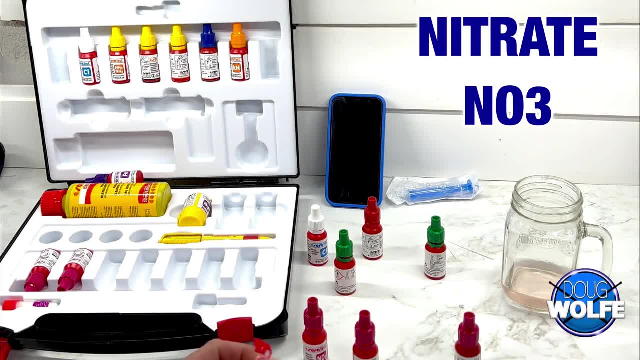 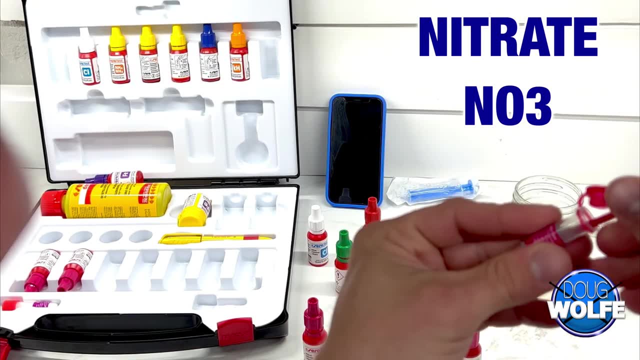 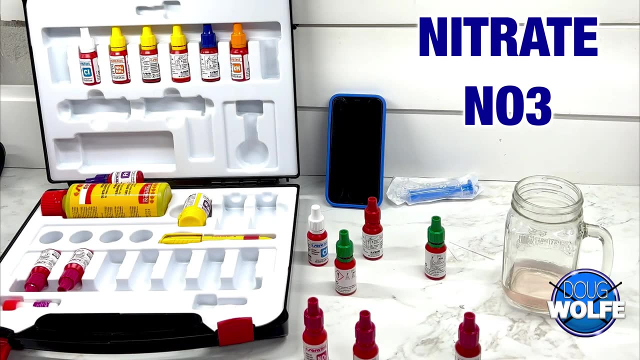 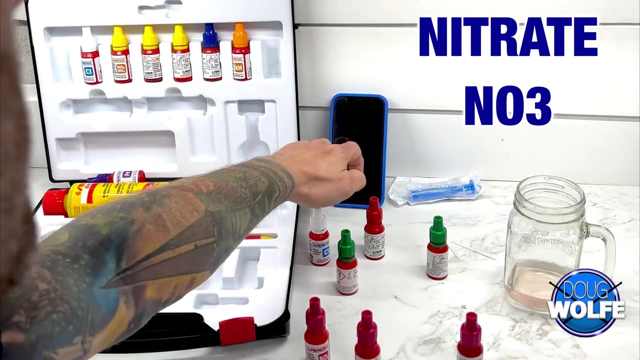 and what we do is take that off. so we're gonna grab- hopefully you can. the camera picks this up. see how it puts a little bit in there. all right, we're gonna add that now we're going to shake for precisely 15 seconds. let's see if this will. 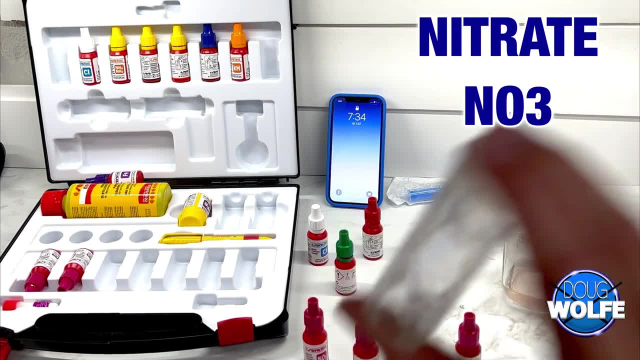 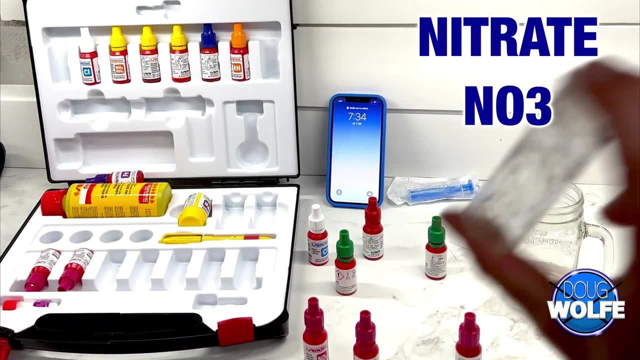 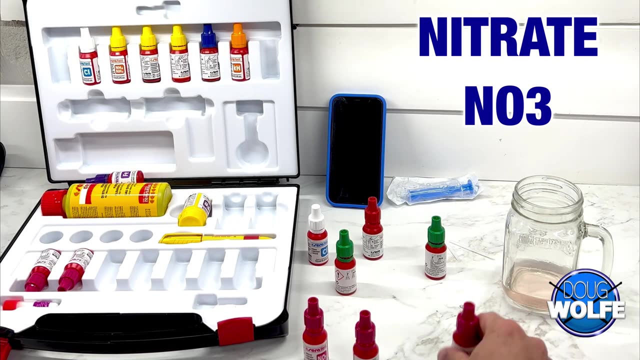 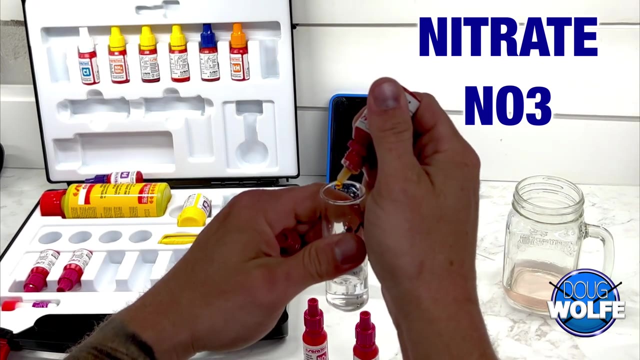 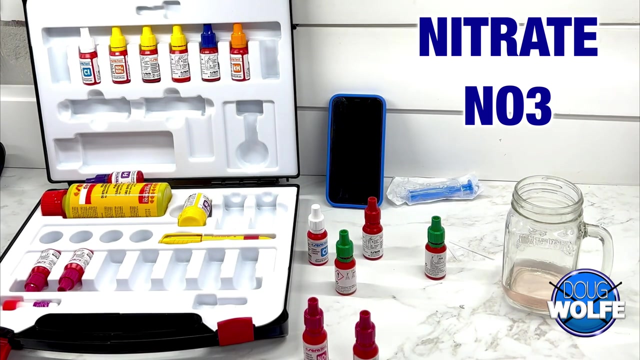 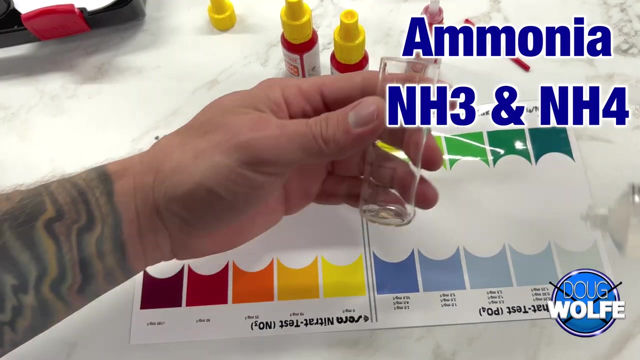 Okay, six drops of the fourth solution: One, two, three, four, five, six, And we are going to shake that until the liquid is distributed evenly, And then we're going to wait five minutes. And, last but not least, actually normally would have done this one first. 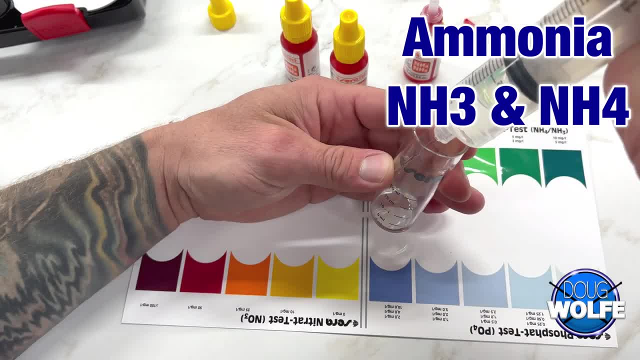 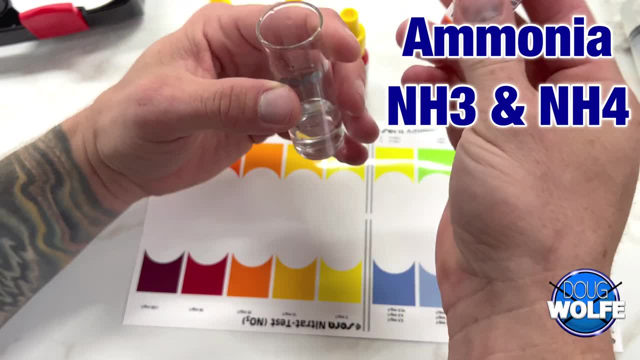 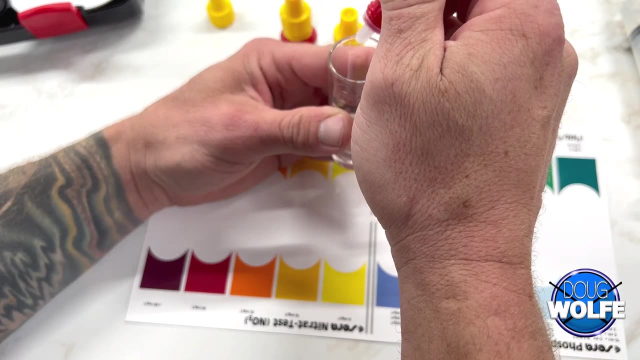 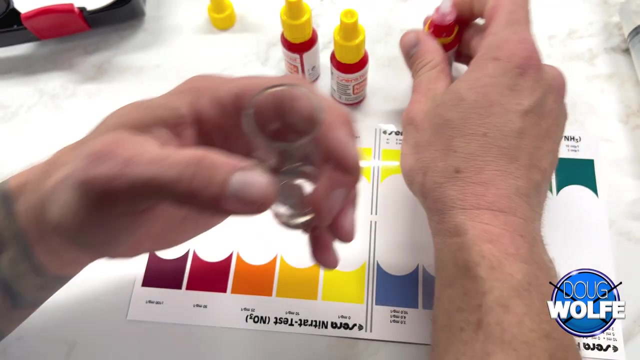 I don't know why I did it last. It's going to be ammonia. Five milliliters for fresh water, five milliliters for salt water. These have already been shaken shook. Six drops: One, two, three, four, five, six. 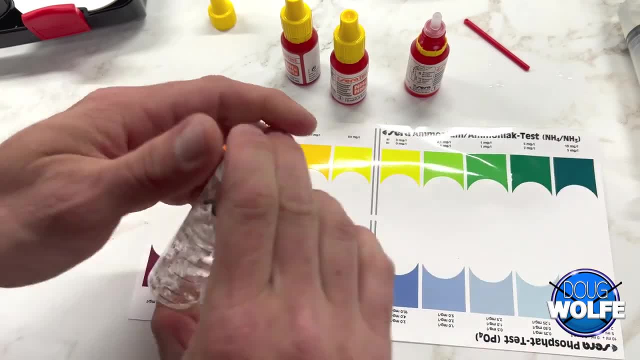 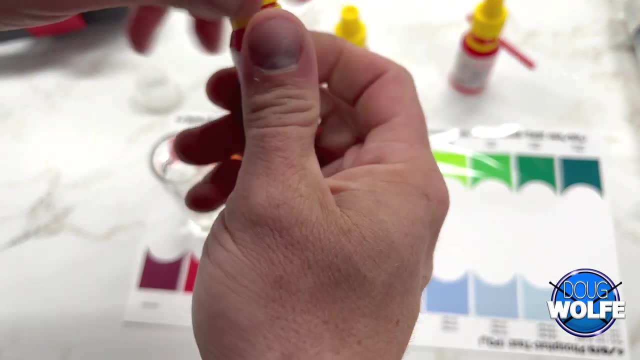 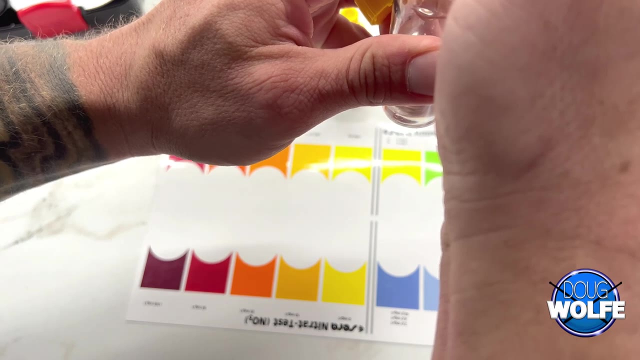 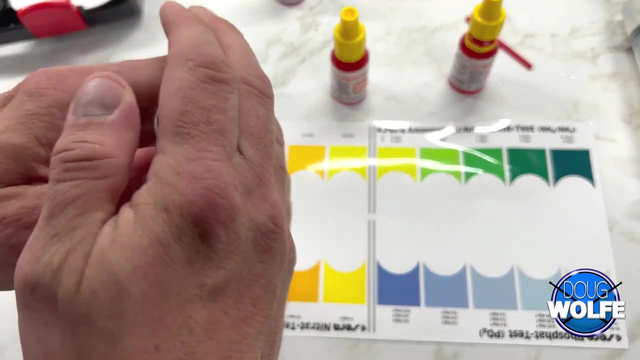 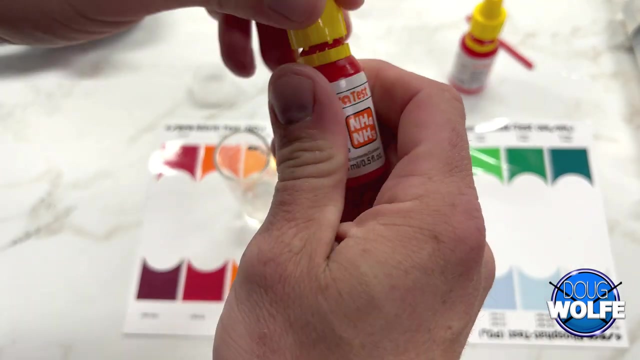 Cap it shake it. Bottle number two: Mix that in One, two, three, four, five, six, Cap it shake it. And, last but not least, 30.. One, two, three, four, five, six. 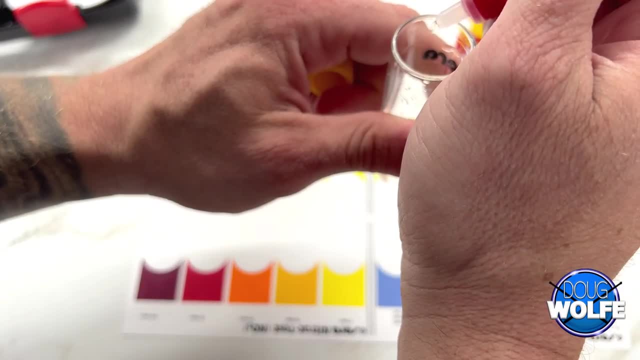 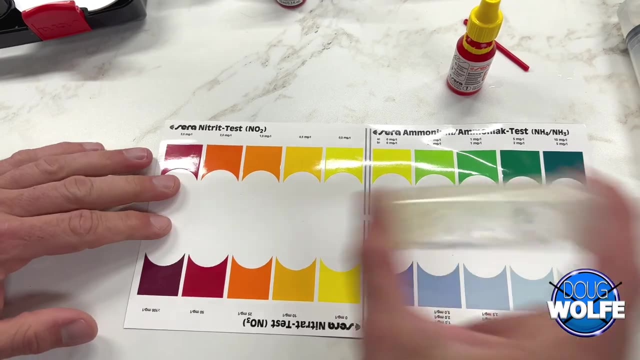 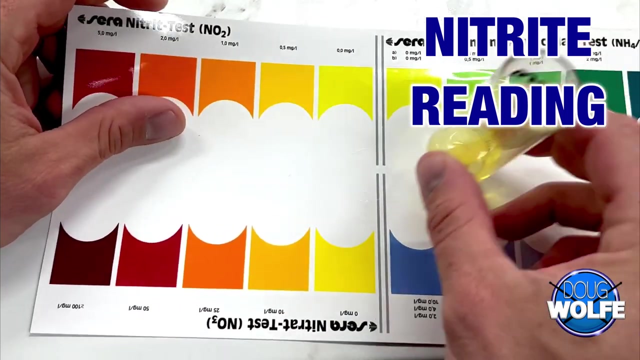 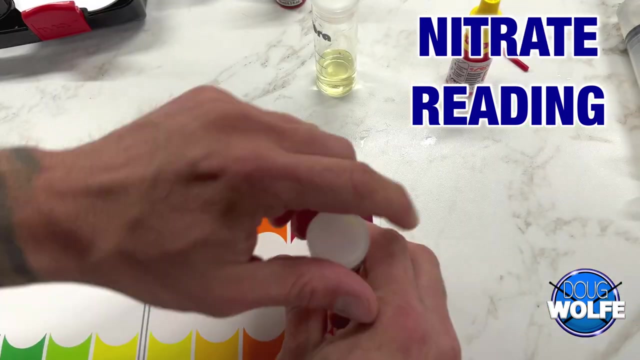 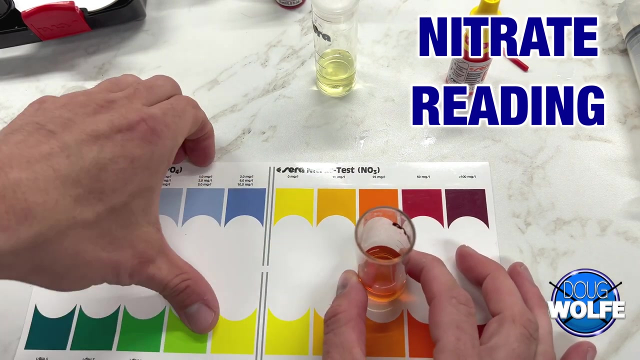 Whoo, That's four. We're going to lips One separate shot, riddle Two. think I hit six there. wait five minutes. hopefully you can see this so you would just move it along the way here. I mean, it's, it's pretty, pretty clear, I guess. 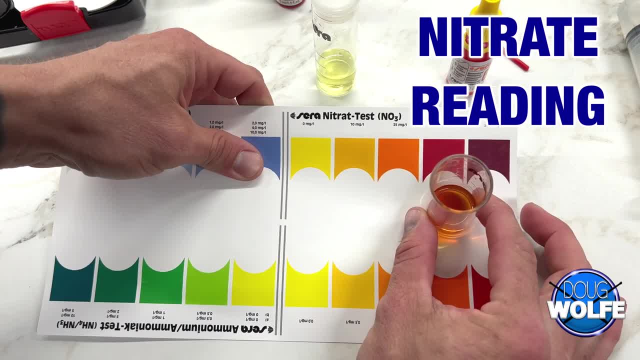 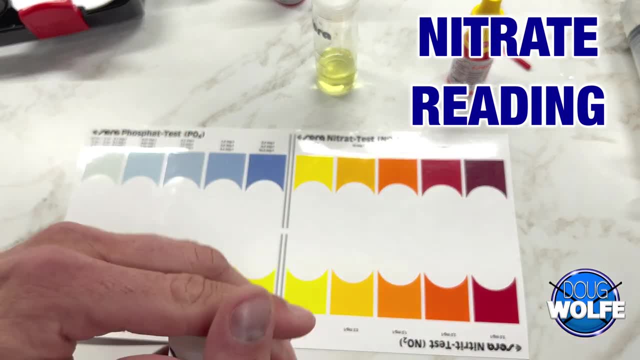 hopefully this camera can see this, but I'm right in here in the 25 range, so not terrible. my tap water here is actually. it varies, but sometimes I get 20 just out of my tap water. so for your ammonia it seems like it could be a little. 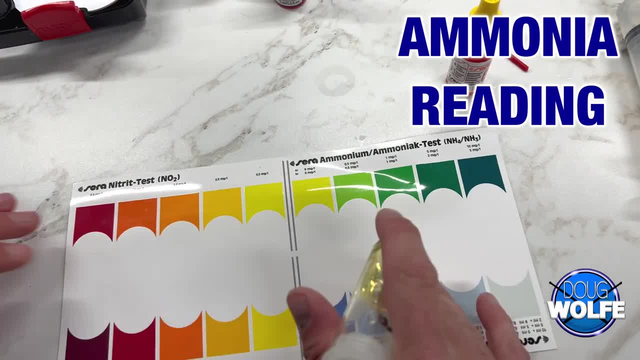 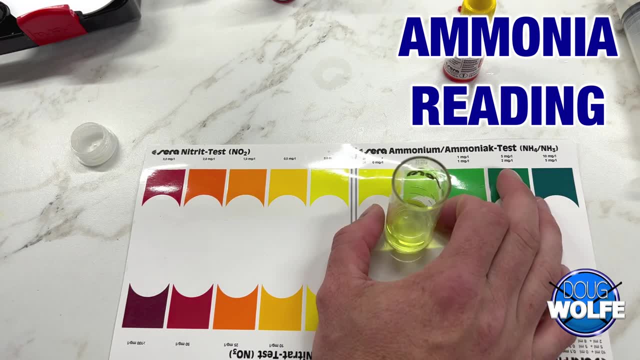 intimidating, but to understand. but it's really not if you break it down. so what we're reading here is your total ammonia, and that is going to be your free ammonia, or your toxic ammonia, which is any ammonia that you have in your tap water, and that is going to be your free ammonia, or your toxic ammonia, or your 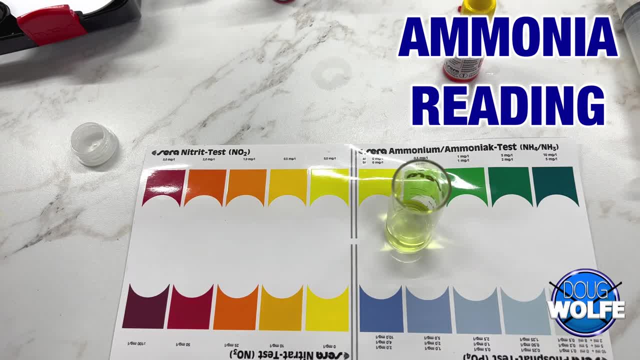 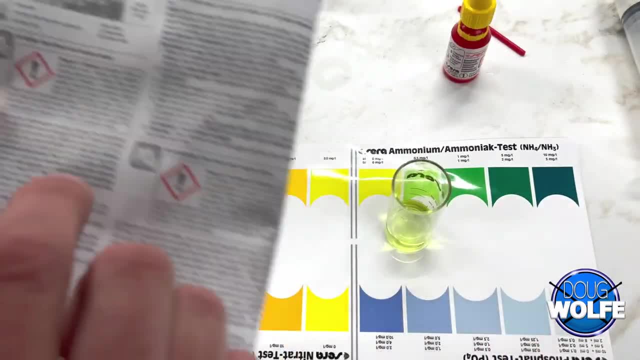 ionized or non-toxic, essentially ammonia, to figure out. okay, what do I have? is my? is this ammonia level toxic for my fish or not? they provide you with this chart here and what you're gonna do is grab your reading off of the far left column. 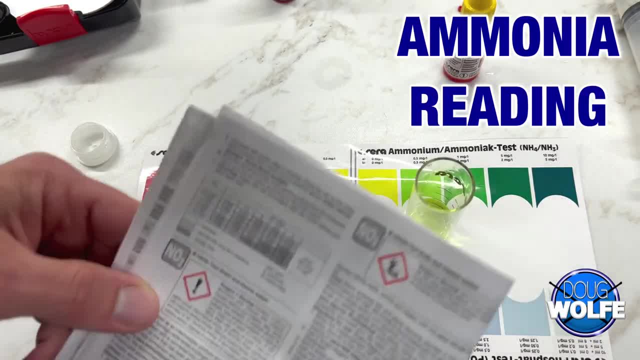 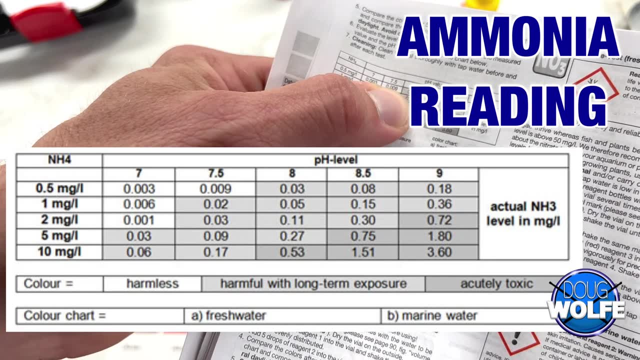 that is based off your color. so say you're at 0.5. and then you're gonna. you need your pH value. so say your pH is 8, you would just go over. so at 0.5. at 8 is a toxic level of 0.03, so that's. 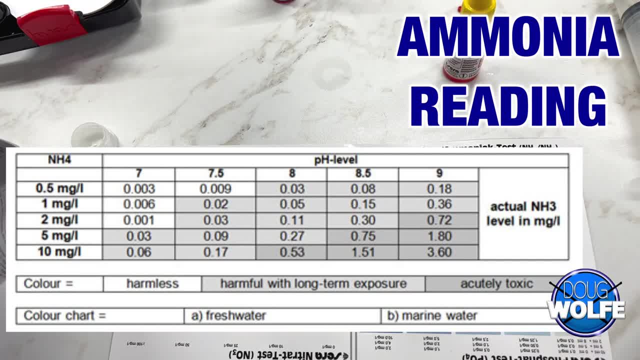 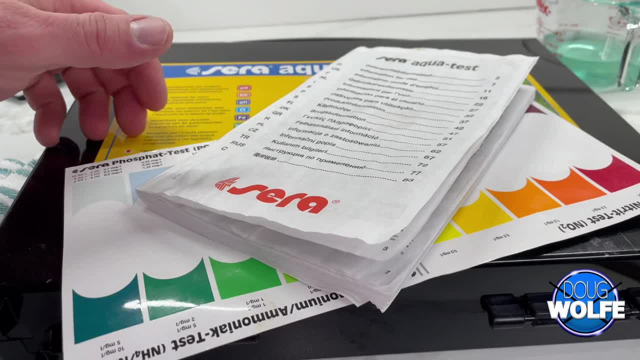 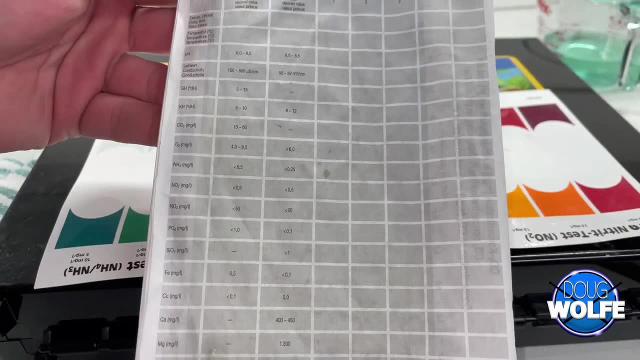 essentially like a stressful level for them, and that's all broke down right here on the chart. as to whether you know your level is something that you need to be concerned about or not. so that is the test kit in a nutshell. I forgot to show you a couple things on the instruction manual. on the back they do have a chart. 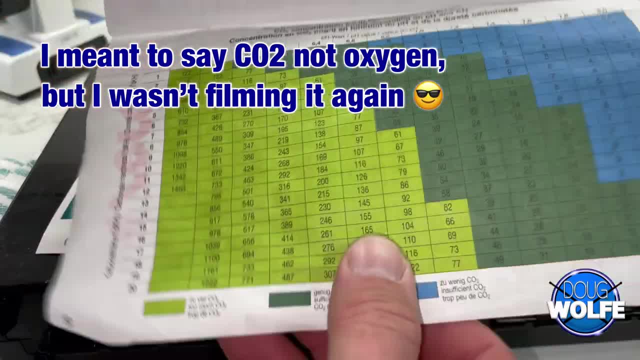 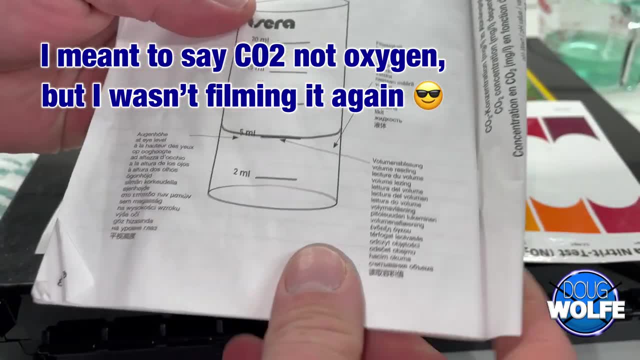 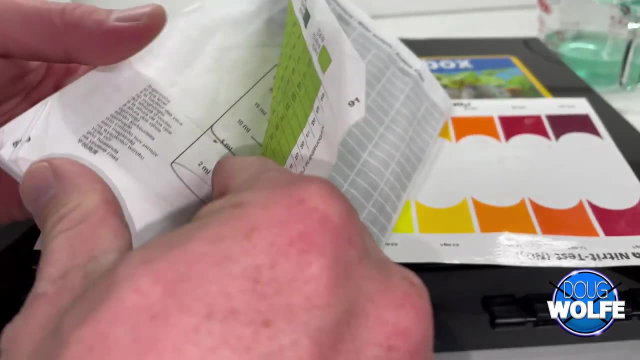 where you can document your readings. in addition to that, they have the oxygen levels for when you get to do your oxygen testing. and then on the opposite page here, if you don't know how to read a meniscus or where that line should be, just some clear instructions on that for you. and also, they do have the ammonia. 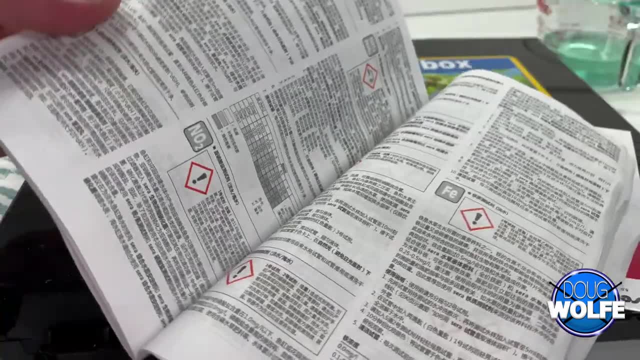 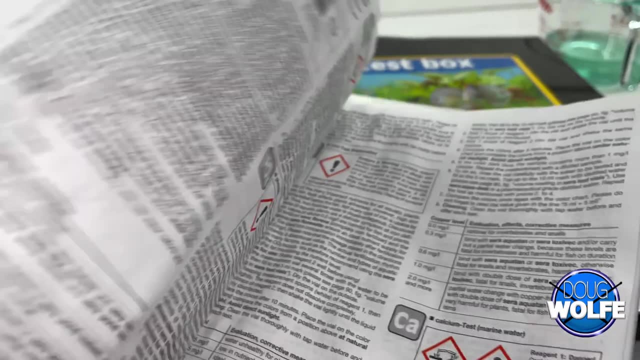 chart in the front as well, and if it's a little, it is a little small to read, so I just print mine offline. you can get a blown-up version of it. it makes it a little bit easier to read. other than that, that's about it, so I 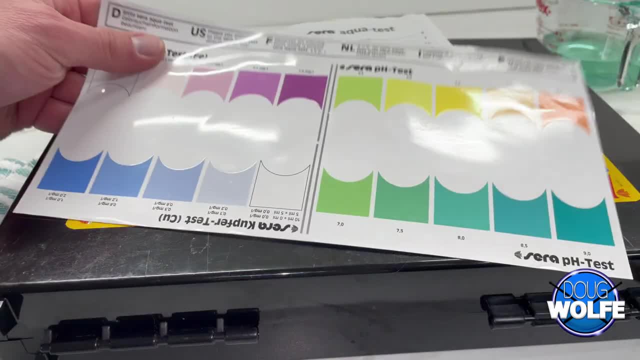 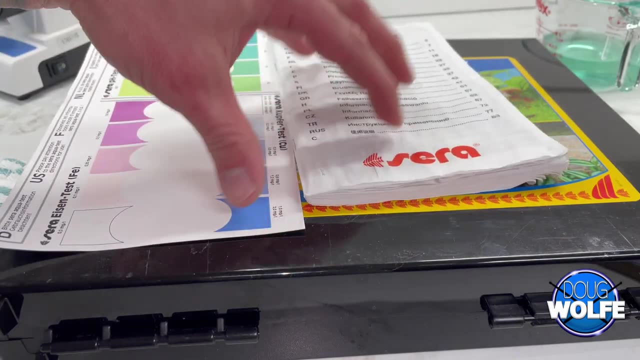 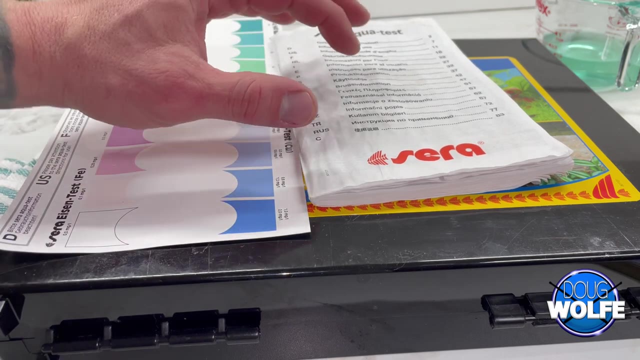 am going to do another video with the hardness testing and I want to grab the oxygen test, a copper test, from Sarah to try those out. and I'm not, you know, endorsed by this company or anything, but I just I like, I like what they have going on. if you go to their website, you can actually create an account, input all.